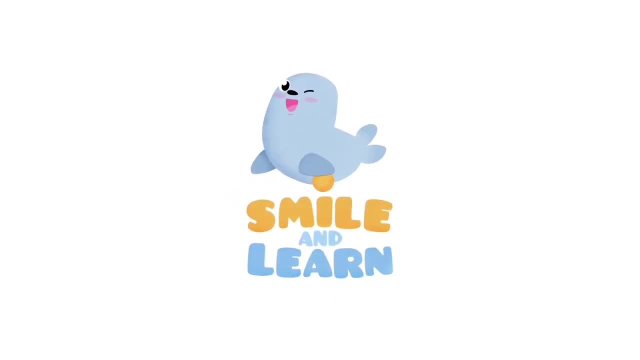 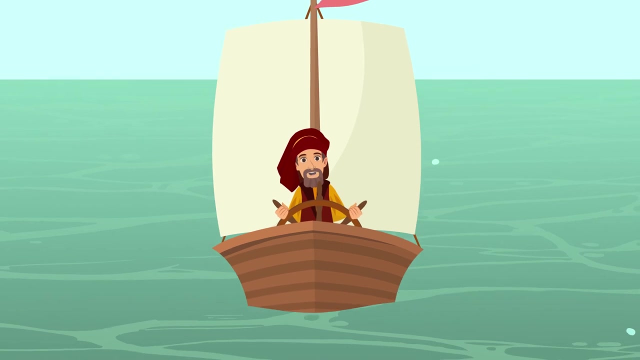 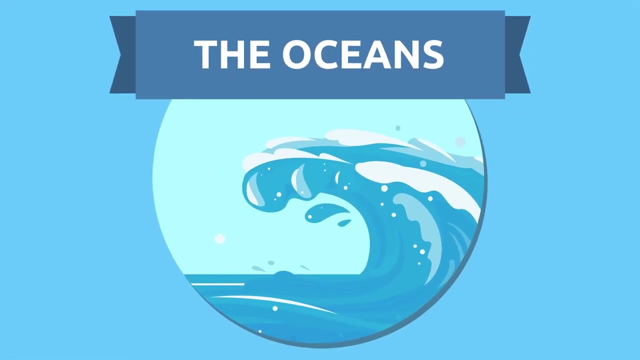 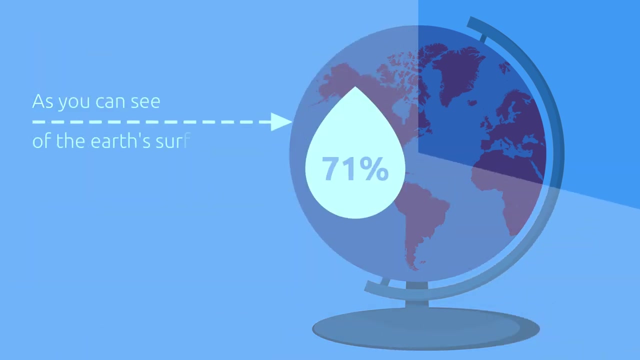 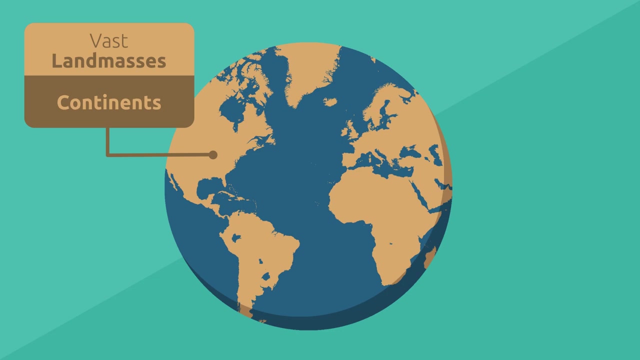 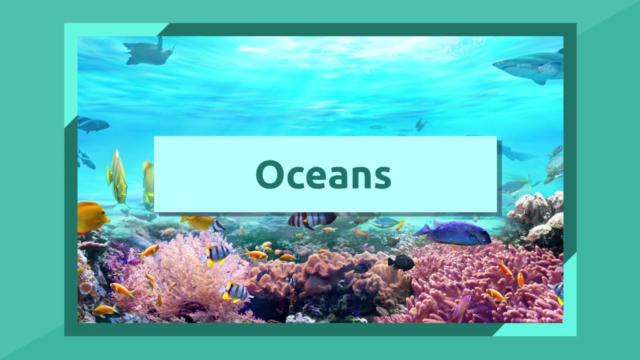 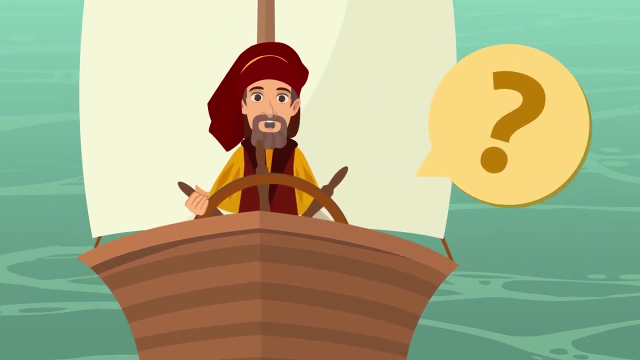 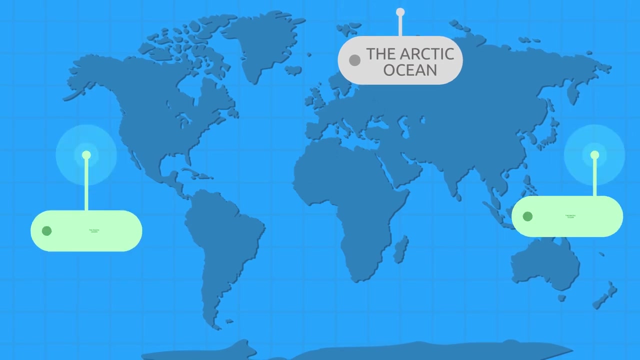 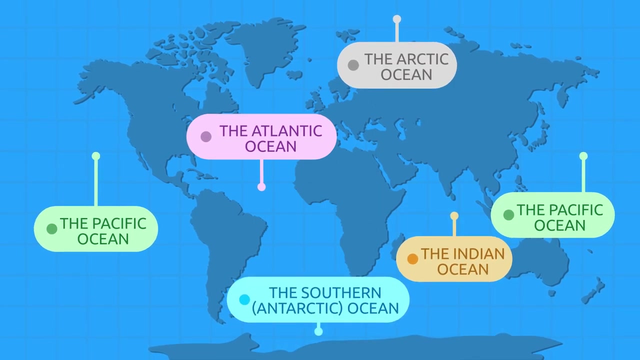 Smile and Learn The vast landmasses separated by large expanses of water. These expanses of water are called oceans. Do you know how many oceans are there and what are their names? There are five oceans on Earth: The Arctic Ocean, the Pacific Ocean, the Atlantic Ocean, the Indian Ocean and the Southern Antarctic Ocean. 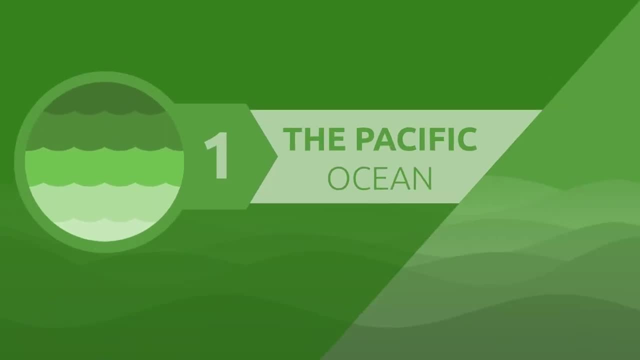 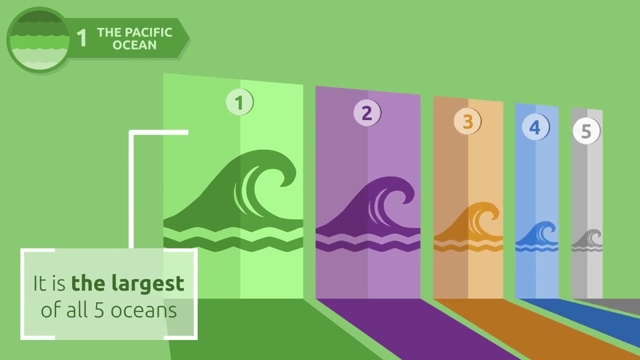 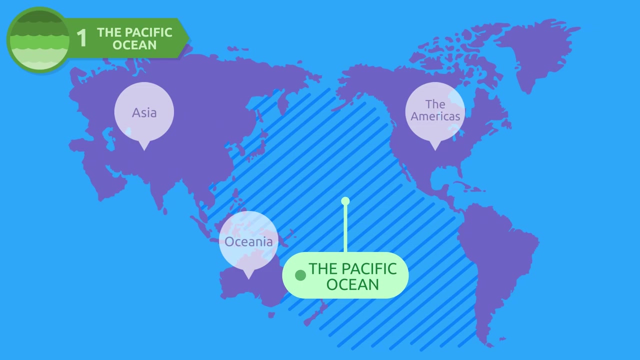 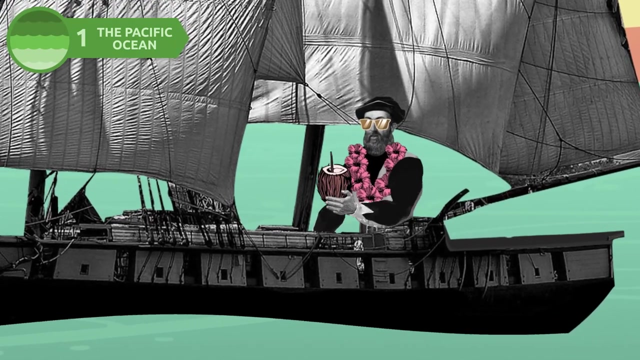 Let's find out more about each one of them. The Pacific Ocean. The Pacific Ocean is the largest of all five oceans on Earth. It stretches from the shores of the Americas to Asia and Oceania. Ferdinand Magellan named it the Pacific Ocean because during his sea voyage, the waters were calm and peaceful. 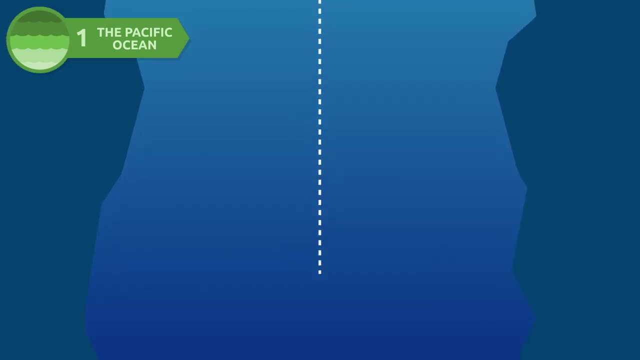 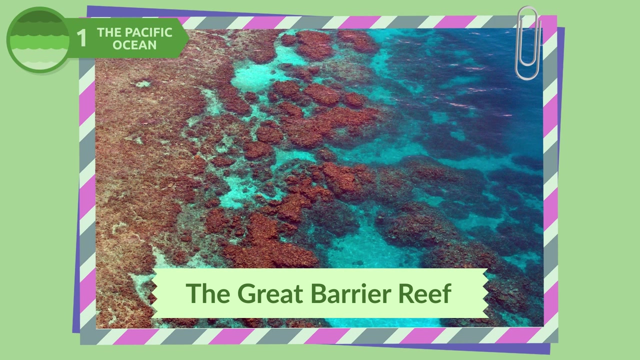 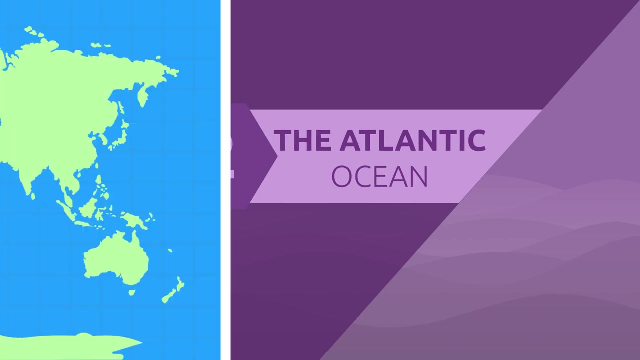 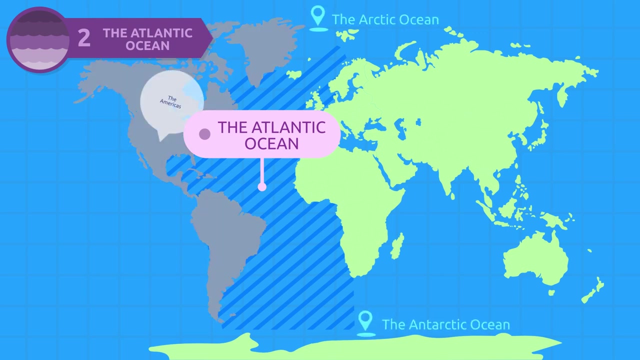 The deepest place on the planet is located here in the Pacific Ocean and is known as the Mariana Trench. Did you know that the Great Barrier Reef is also located in the Pacific Ocean, The Atlantic Ocean? The Atlantic Ocean stretches from the Arctic Ocean to the Antarctic Ocean, bounded on the west by the Americas and on the east by Europe and Africa. 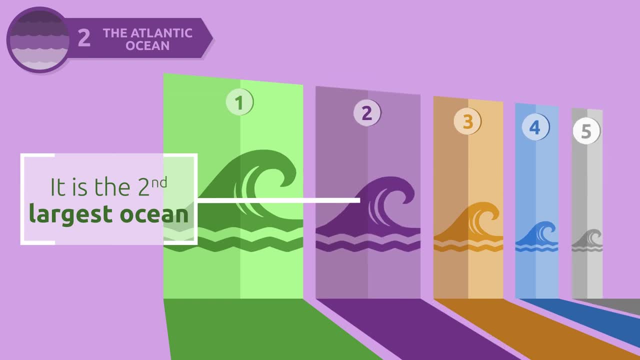 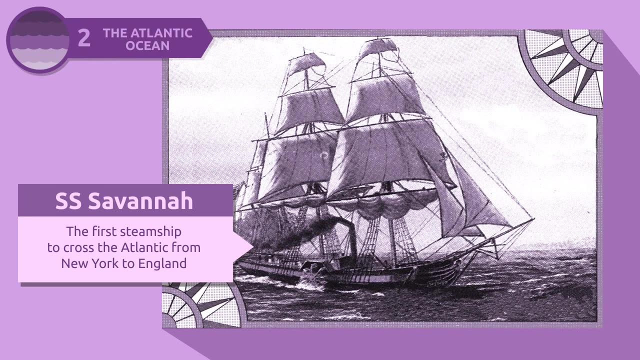 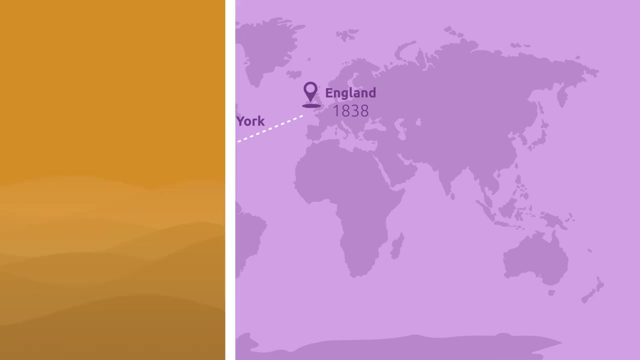 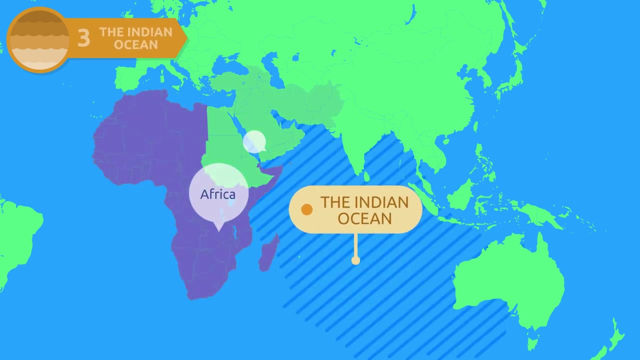 Did you know that it is the second largest ocean on our planet? The first steamship to cross the Atlantic from New York to England was the SS Savanna in 1838.. The Indian Ocean. The Indian Ocean is bounded on the east by Africa and the Middle East and on the south by Asia and Australia. 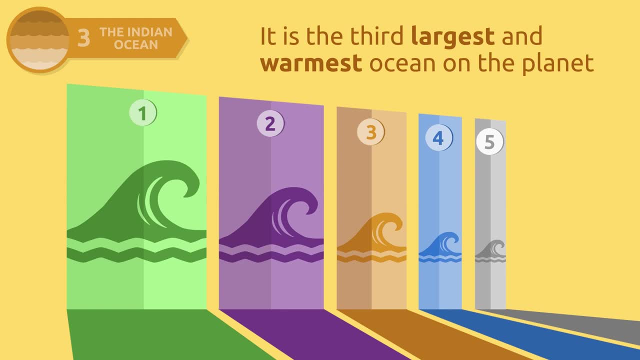 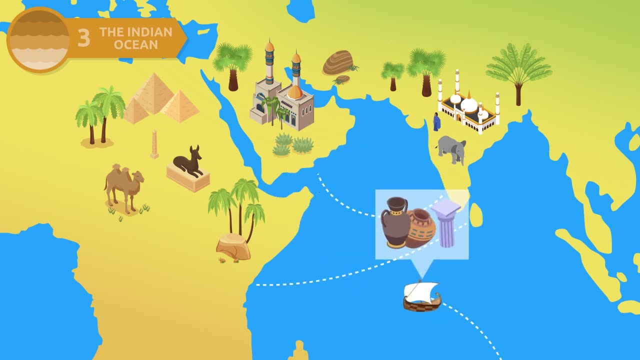 It is the third largest and warmest ocean on the planet. The Indian Ocean is the third largest and warmest ocean on the planet. The Indian Ocean is the third largest and warmest ocean on the planet. In the course of history, due to east-west commerce, the Indian Ocean became an important throughway for transport. 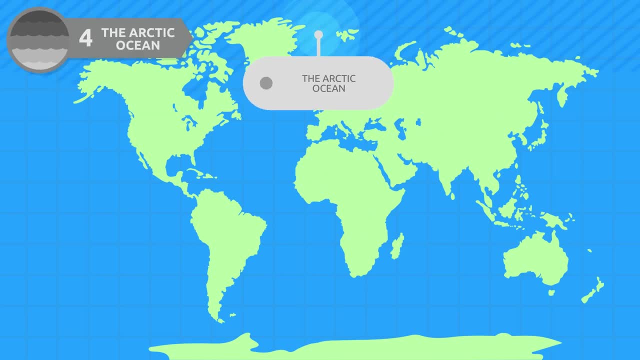 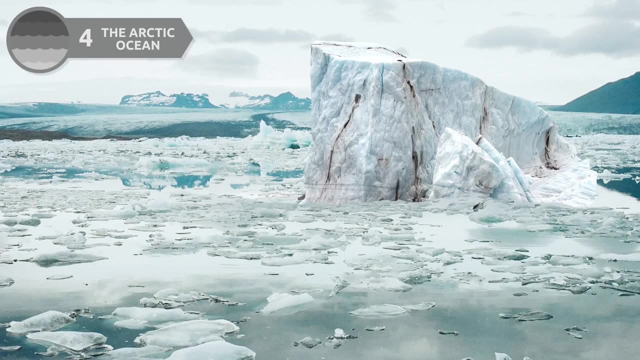 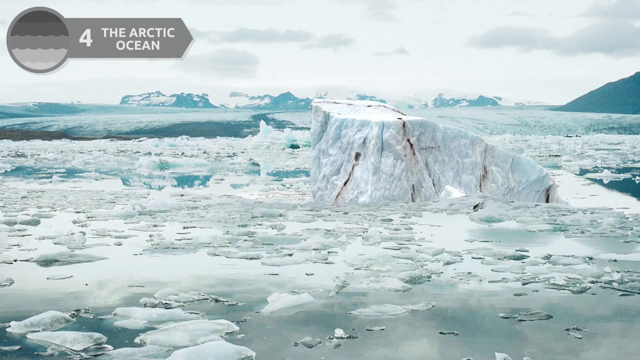 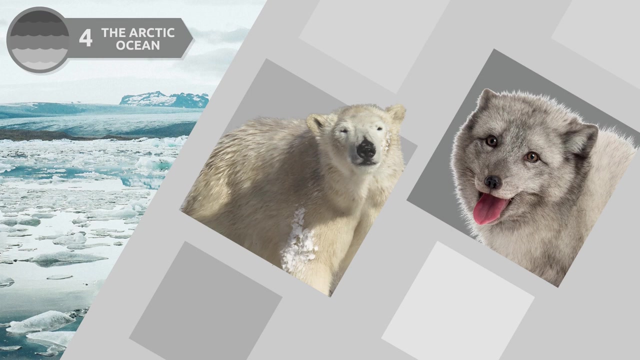 The Arctic Ocean. The Arctic Ocean is located around the North Pole and is the shallowest of all oceans. The largest part of the Arctic Ocean is covered with ice which, owing to global warming, is slowly shrinking. Besides being the smallest ocean, it is important to life on Earth. 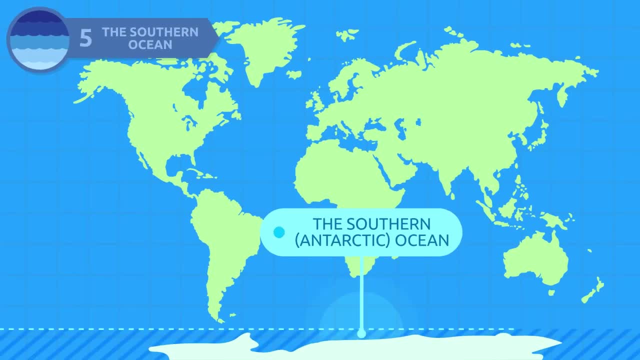 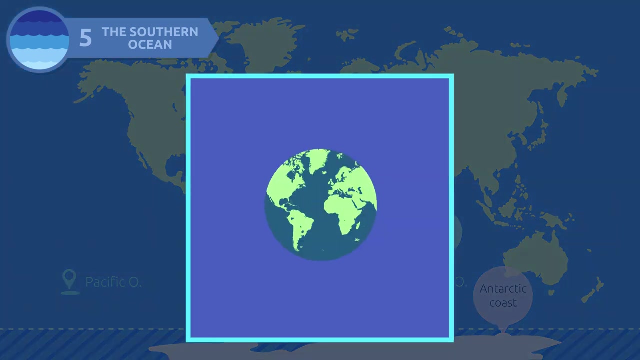 The Southern Ocean. The Southern Ocean, also known as the Antarctic Ocean, is located in the southernmost waters of our planet. It stretches from the Antarctic coast to the Atlantic Ocean, the Pacific Ocean and the Indian Ocean. The Antarctic Circle is marked on maps as one of the major circles on Earth. 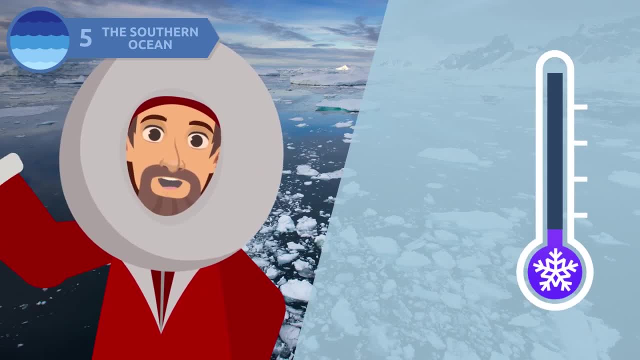 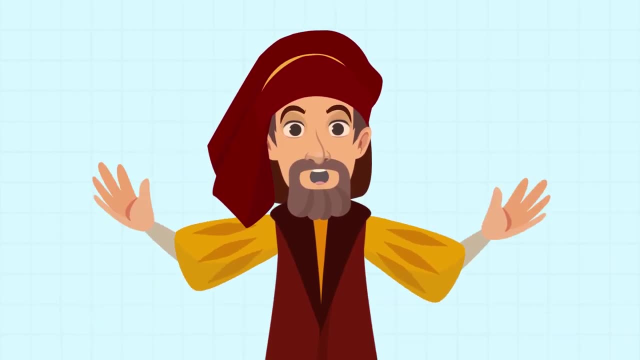 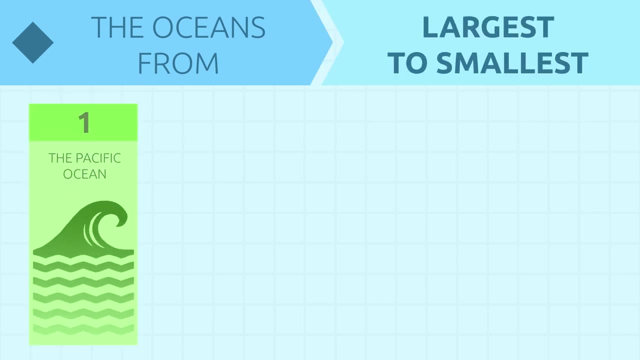 The water temperature in the Southern Ocean is very low, varying from negative 2 degrees Celsius to 10 degrees Celsius. Today, we traveled around the world. As you have seen, the oceans from the largest to the smallest are the Pacific Ocean, the Atlantic Ocean, the Indian Ocean, the Southern Ocean. 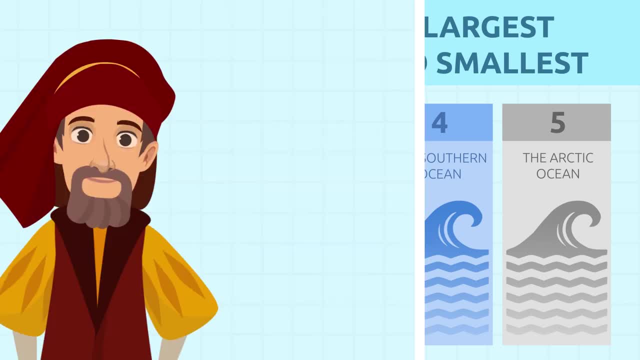 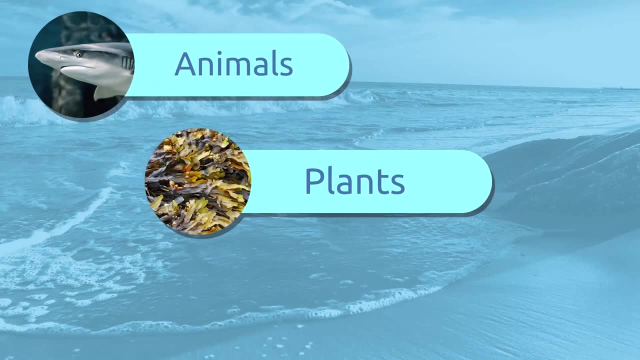 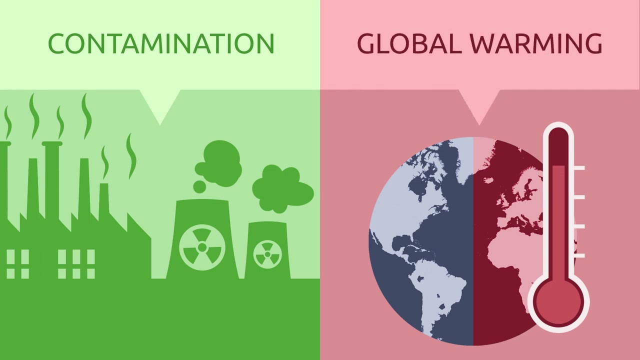 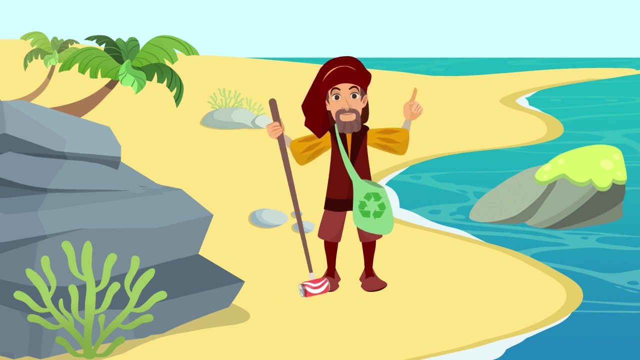 And the Arctic Ocean. Oceans are beautiful places and have a significant influence on our planet. Numerous species of animals and plants and many types of ecosystems can be found in the oceans. Unfortunately, contamination and global warming threaten ocean life. That's why it is really important to look after the oceans and protect the environment. 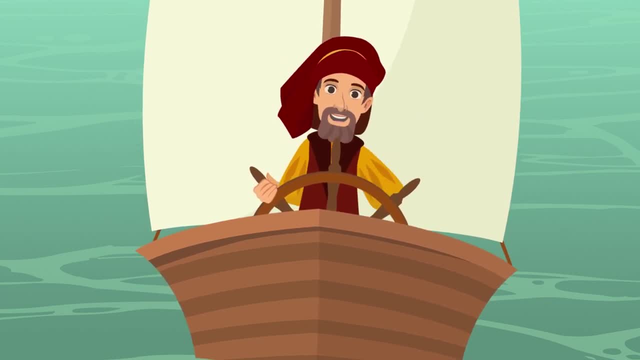 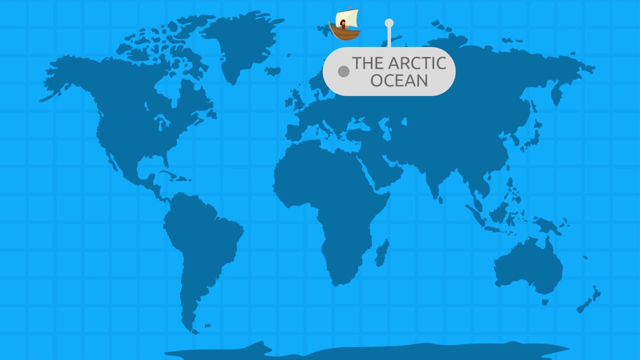 This has been a sensational trip. Thanks for watching. We learned everything about the five oceans on our planet. Can you remember all of them? The Arctic Ocean. The Atlantic Ocean. The Southern Ocean. The Indian Ocean. The Pacific Ocean. Well done, explorers. 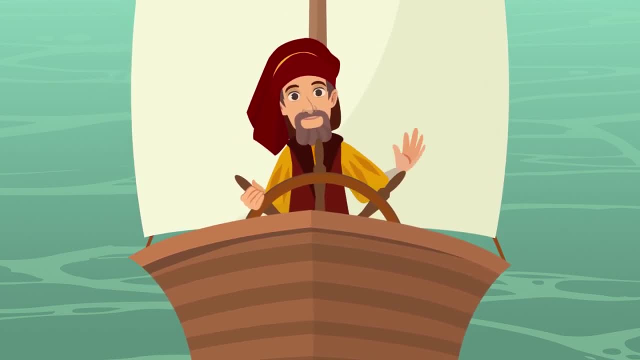 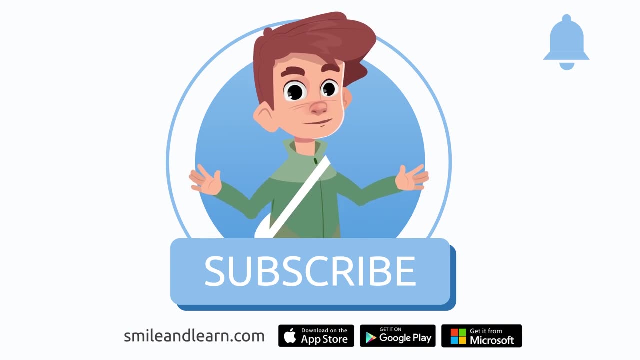 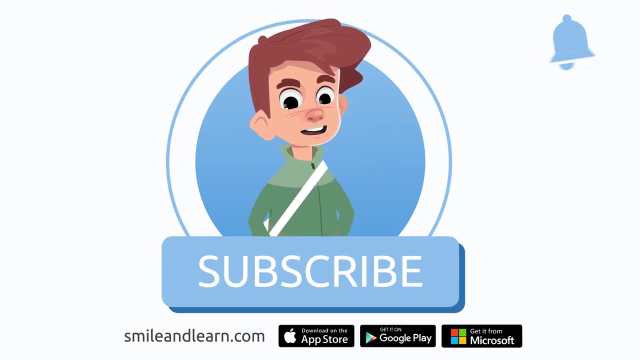 See you soon for our next exploration. We've learned so much in just one video. Did you know there are many more videos? Imagine how much you could learn. Subscribe to the Smile and Learn educational channel to learn and have fun at the same time.